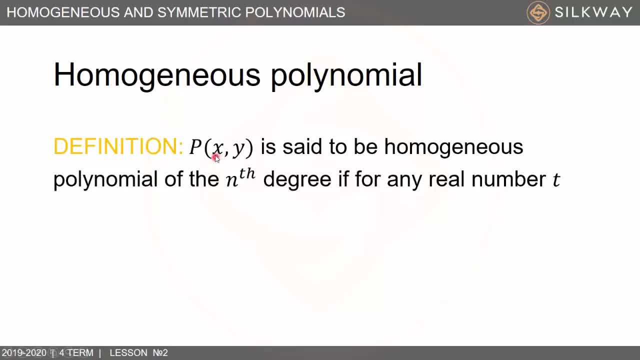 polynomial with variables X and Y is said to be homogeneous, polynomial of the nth degree if, for any real number, T, this expression is correct. In other words, polynomial is nth degree homogeneous polynomial if the degrees of its terms are equal. Okay, let's look to the example. 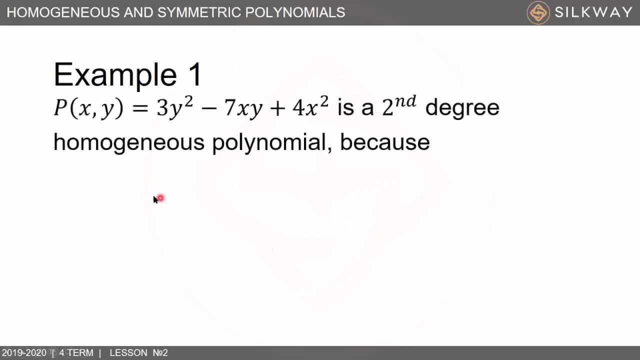 first example, this is our polynomial, and let's see degrees of each monomial. First monomials degree is 2, seconds is also 2, because 1 plus 1 is 2 and third is also 2.. Okay, and from definition we can say that this is: 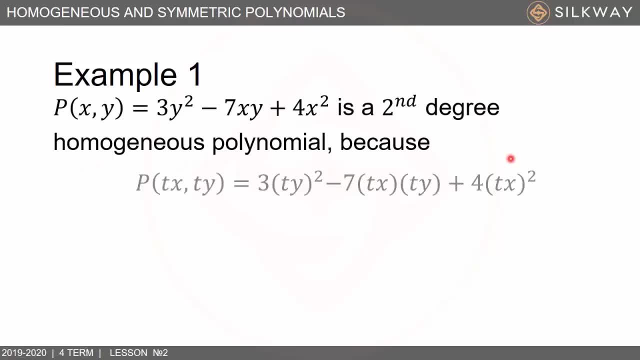 polynomial is homogeneous. And then let's prove it. Okay, We multiply by T each term, and if we open brackets, here, square, this will be 3 T square, multiplying by Y square, and here's also T and T multiplying will be T square and here's, if we open bracket, will be this one, and then 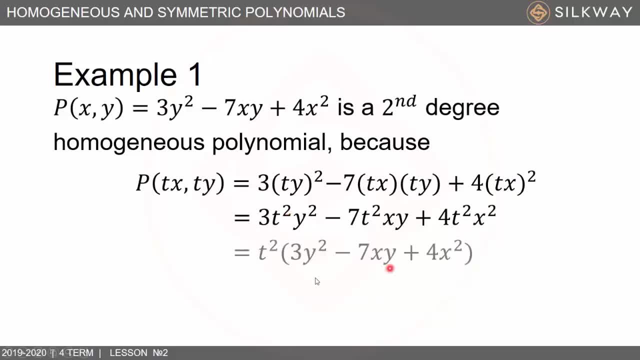 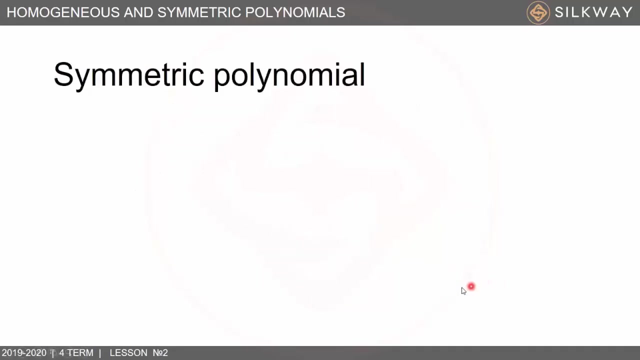 we take T square out of a bracket and we will have a square And we will have this polynomial, Our initial polynomial. Okay, and we can write this like that. From definition we can say it's a homogeneous polynomial. Okay, we prove it. Then what is symmetric polynomial? 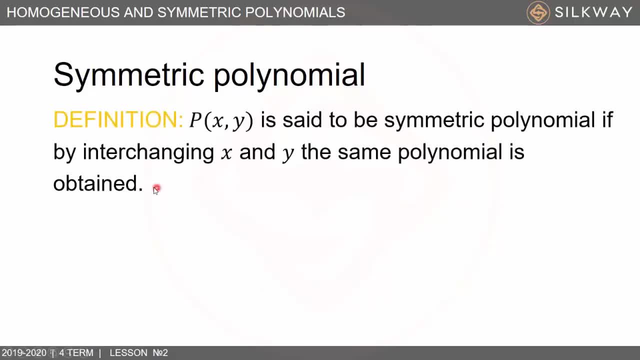 polynomial is said to be symmetric polynomial If, by interchanging all exchanging X and Y, Then what is symmetric polynomial? Polynomial is said to be symmetric polynomial if, by interchanging or exchanging X and Y, the same polynomial is obtained. okay, let's look to the example. 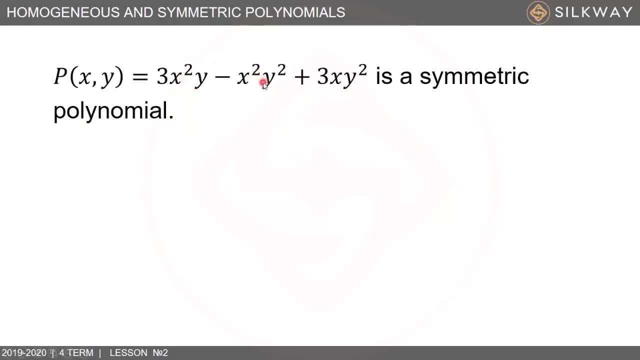 three x square, y minus x, y x square, and multiplying by y square plus three x, multiplying by y square, is a symmetric polynomial. okay, look at this. if we exchange, if we interchange, x and y, what will be? three y square, x minus y square, multiplied by x square.